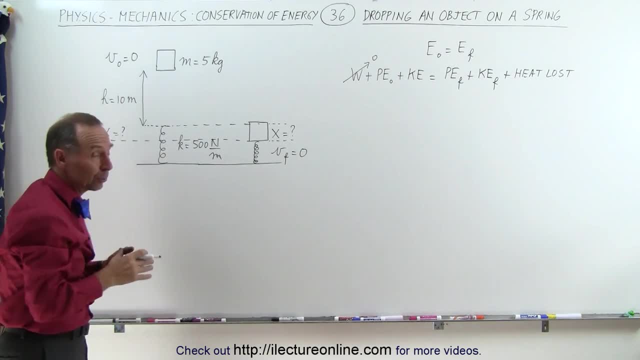 plus we have an additional distance which we don't know yet. it's equal to x, and so we can say that this is the total height of the object. so h total. h total is simply equal to h plus x, which means that the initial potential energy it has. 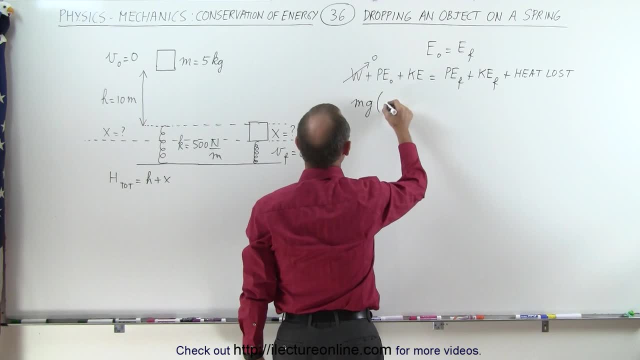 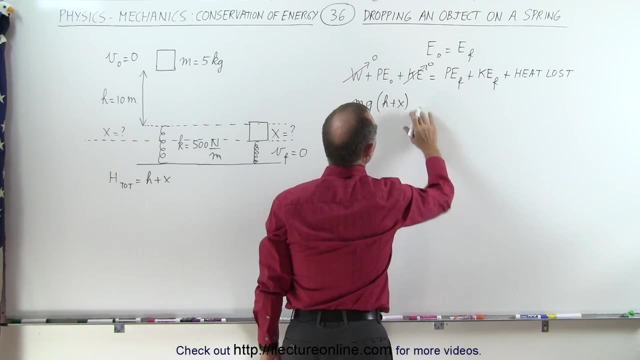 is equal to m times g times h plus x, Kinetic energy is going to be zero. Not add that, because of course it's not moving initially, Then when it gets to its final resting place, and of course, if we then continue with the time, the 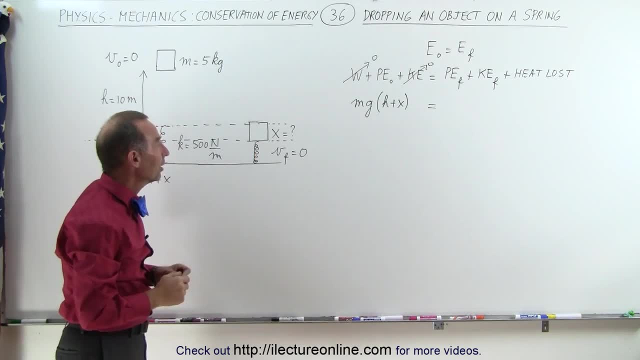 object would bounce back up because of the energy stored in the spring, but at least this would be the final position for our problem and therefore the final potential energy would be the energy stored in the spring, and that is going to be equal to one half the spring. constant times x squared. 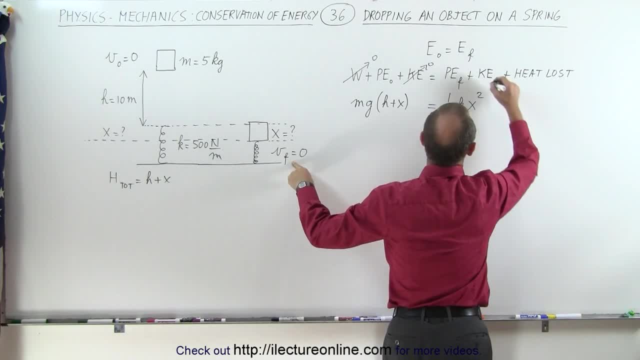 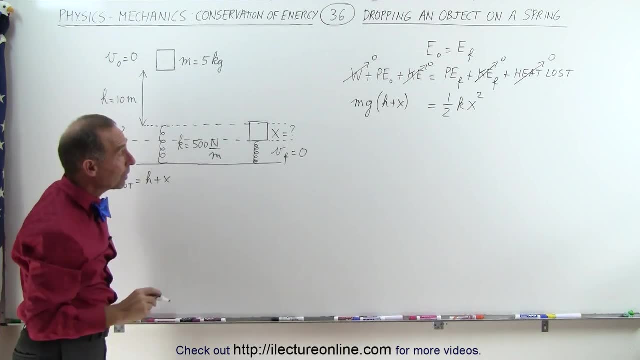 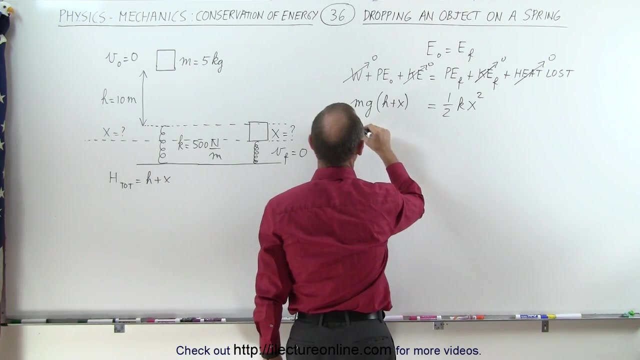 There's not going to be any kinetic energy at the end, because its velocity will be zero and there's no friction. so there's no heat loss due to friction. What we have to do here is take that equation and solve it for x. So let's go ahead and multiply this out. get rid of parentheses first, So we get mgh plus mgx is. 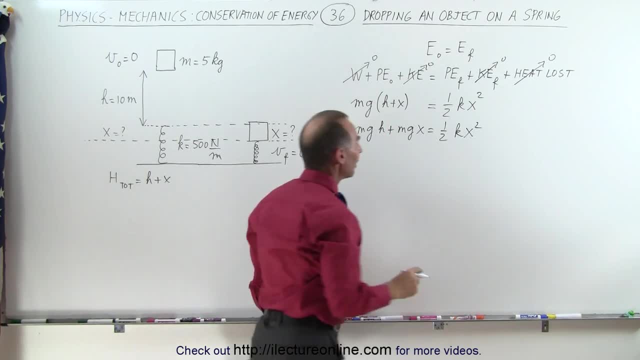 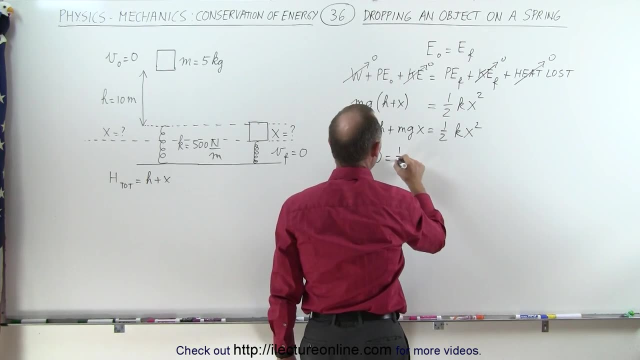 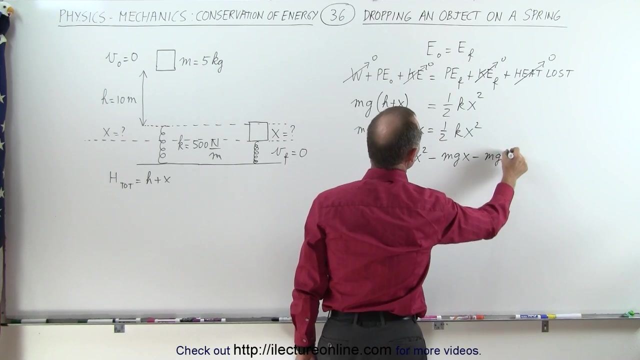 equal to one half kx squared, and it looks like we're going to end up with a quadratic equation. So let's move it around. Let's move everything over to one side. So I have: zero is equal to one half kx squared, minus mgx, minus mgh. Now let's play in the numbers so we can actually solve. 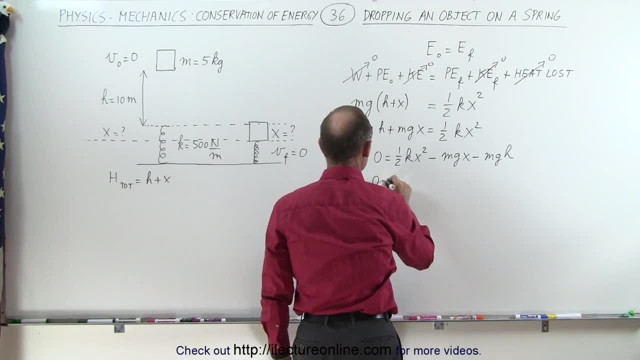 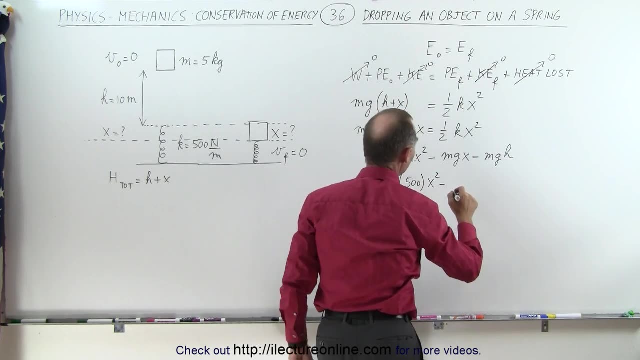 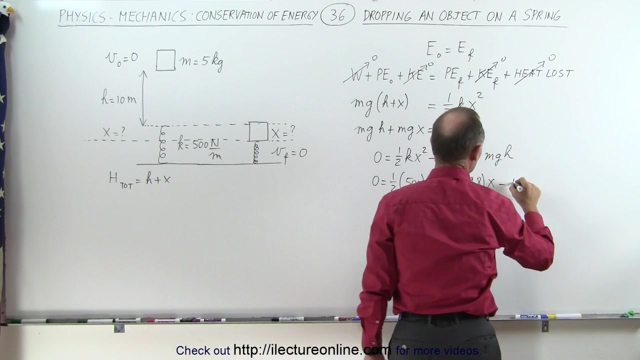 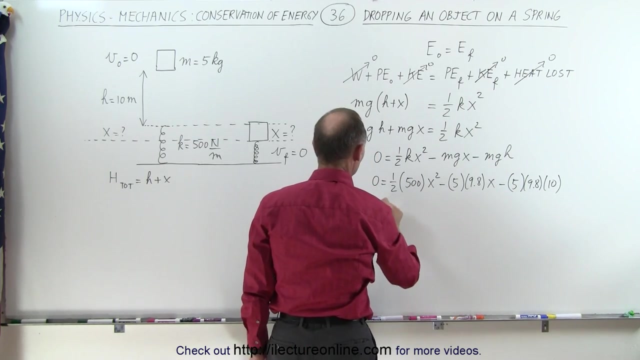 that quadratic equation We end up with: 0 equals one half times k, which is 500 times x squared minus m, m is 5, g is 9.8 times 2.8 times 9.8.. x minus m, which is 5g, 9.8, and H is equal to 10. so simplifying that, we get 0 is. 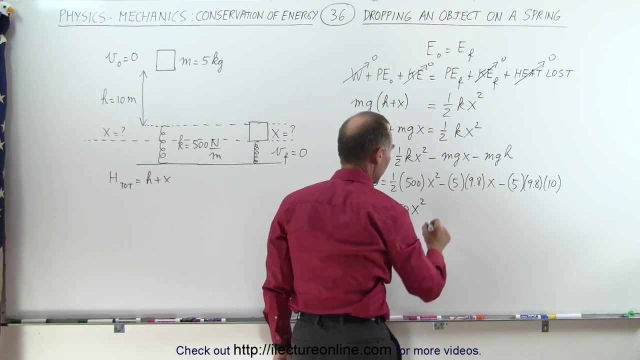 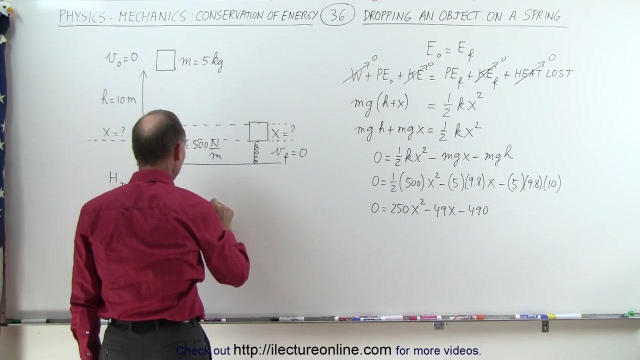 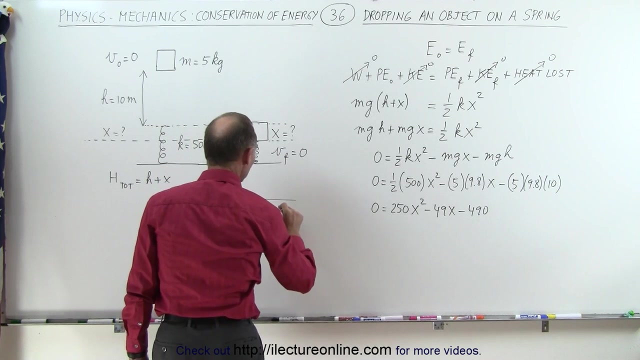 equal to 250 x squared minus 49, X and minus 490, and that's the quadratic equation that we can solve. so X equals minus B, which is 49 plus or minus the square root of 49 squared B, squared minus 4 times a, which is 250 times C. 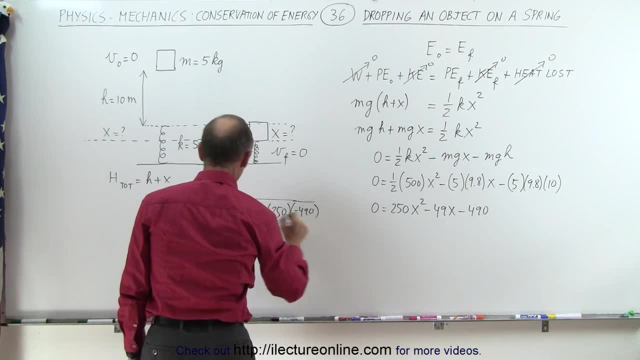 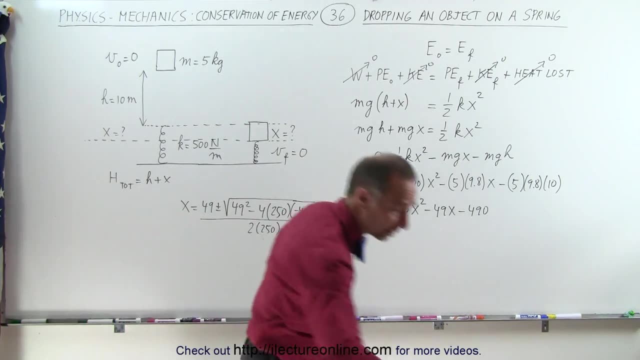 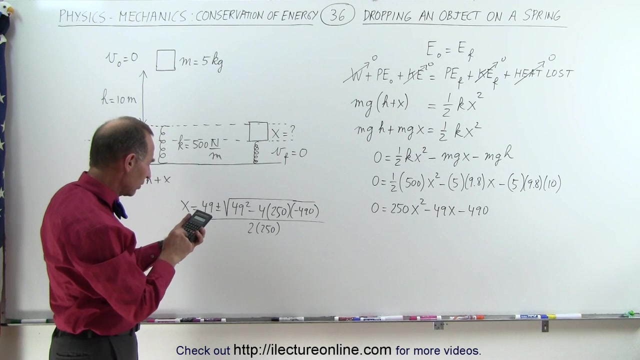 which is a minus 490, and the whole thing divided by 2 times a which 2 times 250. alright, now we're ready to solve that using our calculator. starting with what's inside the radical, we have 4 times 250 times 490. notice that we don't have to do that with the root. here we have 4 times 250 times 490. notice. 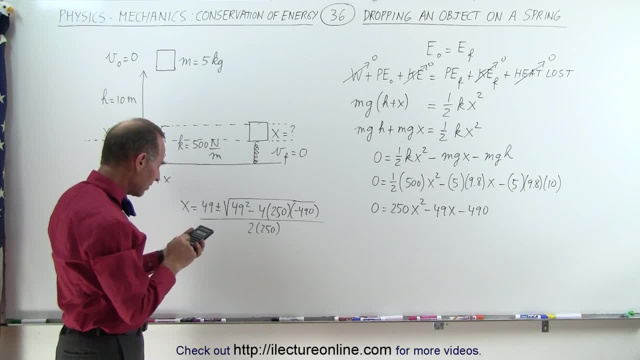 that we don't have to do that with the root. here we have 4 times 250 times 490. notice: the negative sign will cancel out that negative sign. we add to that 49 squared and then we take the square root of that and so this ends up being x is equal to 49. 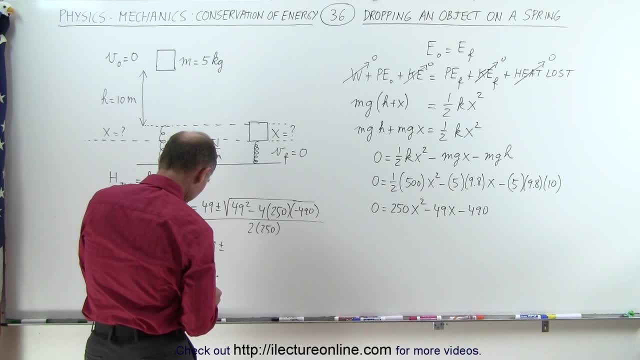 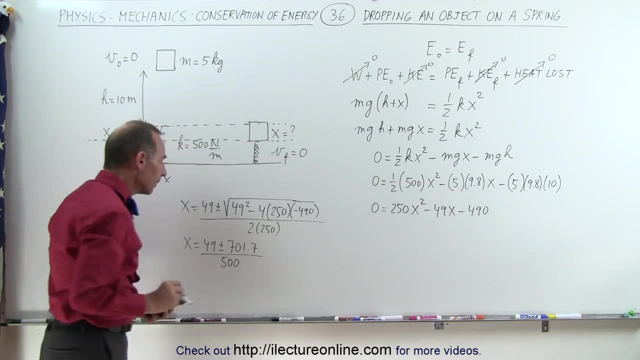 plus or minus the scope, plus or minus not the square root: 701.7 all divided by 500.. All right, so I don't think the negative is one possible answer, because x would then be in negative distance and we can only have a positive distance here. so that means only viable solution.